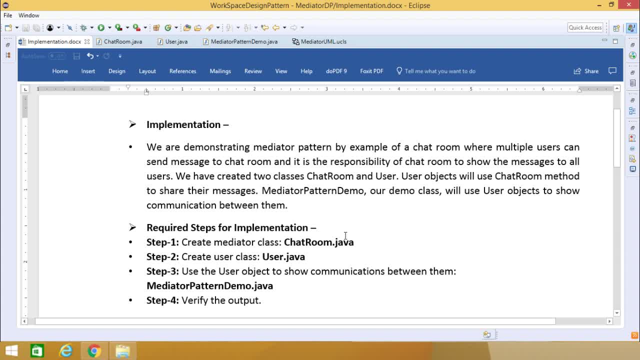 one is the chatroom, another one is the user, and user objects will use a chatroom method to share their messages. Mediator pattern demo is our demo class andwill use user objects to show the communication between them. So this is about implementation of this mediator. 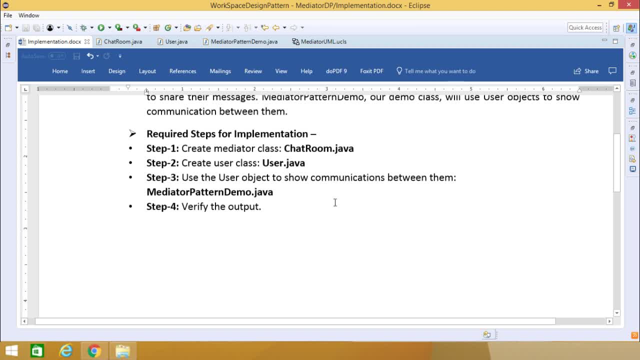 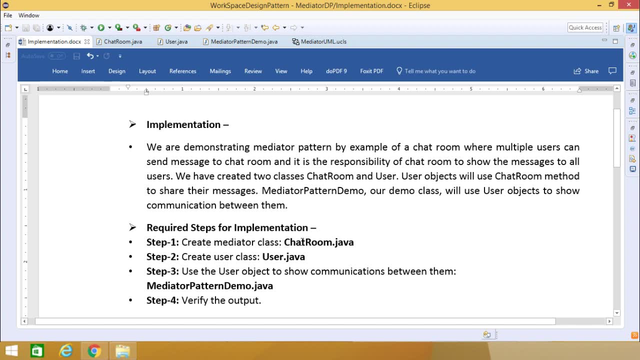 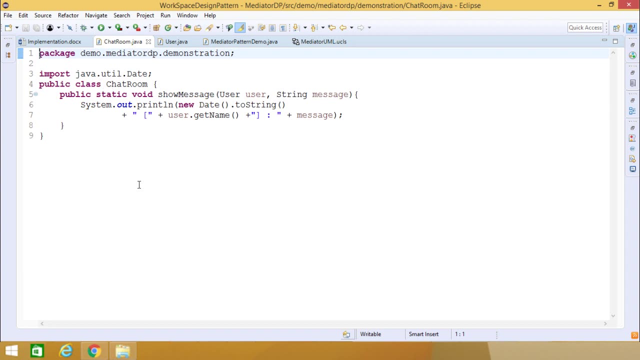 design pattern pattern. so let us go through some certain number of steps. so step one: create mediator class. that is our chatroomjava. so step one: create mediator class, that is chatroomjava. so here we are having this chatroomjava. this is a public class chatroom which is having one public static. remember this. 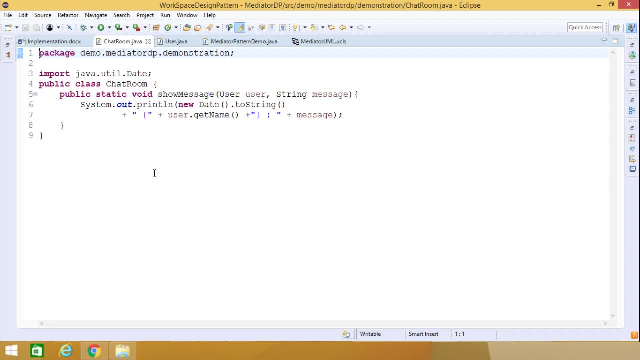 one. it is a static method: void show message, which takes the user and the string message as input parameters, and then systemoutprintln, where having this date is getting printed, then username is getting printed and the message is also getting printed. so in case of chatroom class, we are having 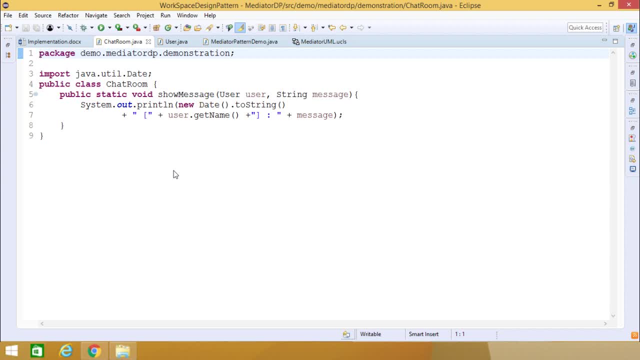 only one static void show message method, which takes the user object as input argument. another one is the string, a message, as input parameter. so now we are having this: systemoutprintln date is getting printed, user get name is getting printed and the respective sells message is getting printed. okay, now what about the user? so this is our user we are having, so 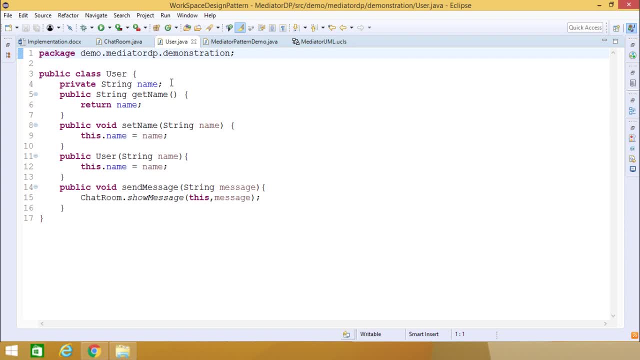 user is having one name, so there is one instance variable. we are having string name, so get name will return this name, so get name return string set name will take one string as input argument which will be assigned to this name instance variable and we are having this user. that is. 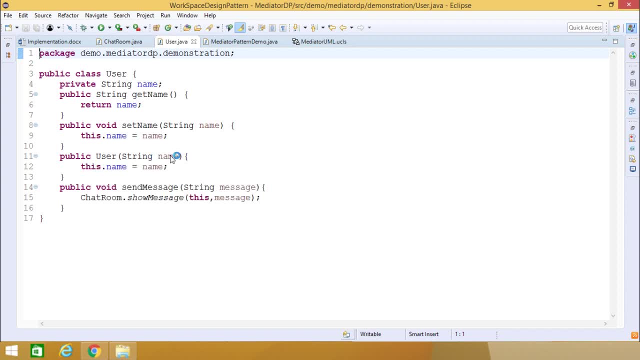 our constructor, which will put this value input argument name to this particular, this dot name. so input parameter name will be assigned to this, this dot name. so we are having this send message. so this is one of the methods in this user class and which takes a string message as input argument. 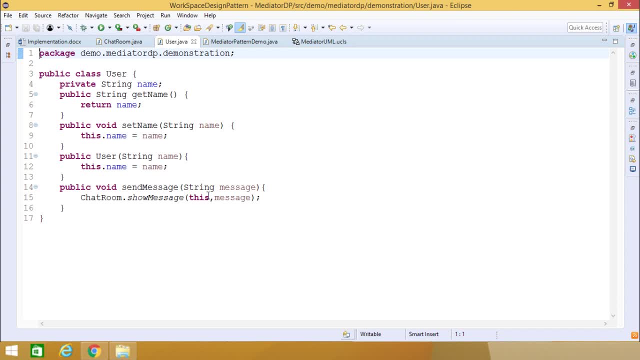 so now we are having this chatroomshow message, this comma message, so chatroomshow message. you can easily find that chatroomshow message will take one user and this message as input argument. so now here we are having this at this and the message will be passed to this chat. 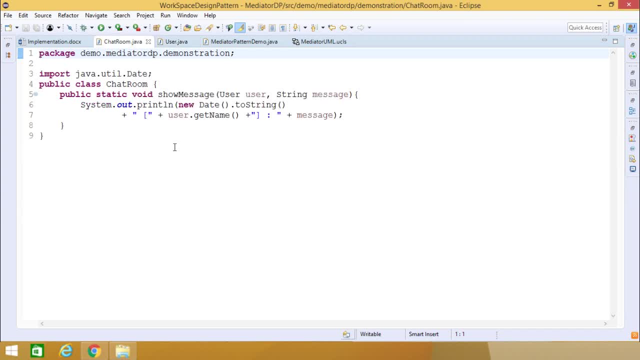 roomshow message. so now, after discussing this chat room, you can easily see that what is the code in chat room there is a class. user is also another class. you can observe its code and now we are going for our demo class, that is mediator pattern demo. so here you see, we are creating one. 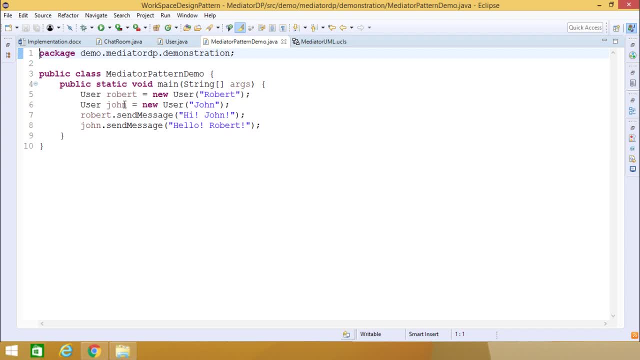 user robot user object. another one is user john. there is a user object is equal to new robot and you are having this new user john. so using the constructor, we are initializing this respective user here. so the name is a instance variable and that is getting initialized with. 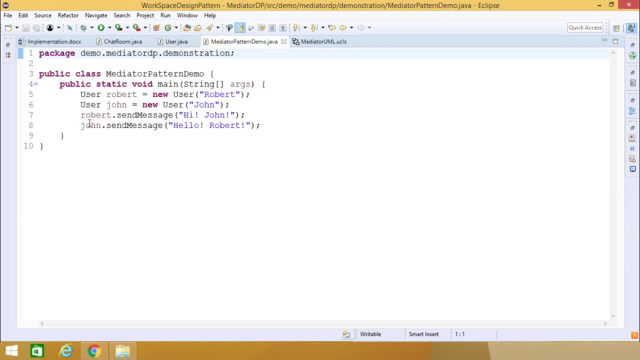 this name string, whatever we have passed. and now we are going for robot dot send message. hi, john and john dot send message. that is a hello robot. so what will happen? we can come to this user- the send message function is there- which will be calling this chatroomshow message method. so 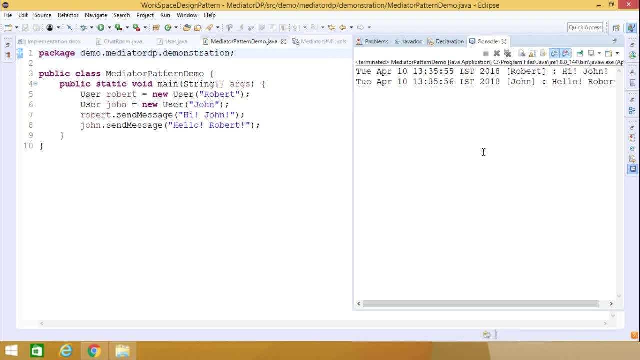 now let me execute my code. you can easily see that this hi john and this hello robot. we passed these two arguments separately in two send message methods: robot dot- send message and john dot send message. robot and john are the user objects. so now you see, this is the respective. 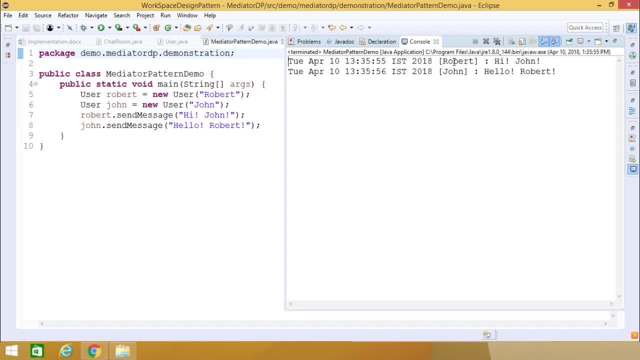 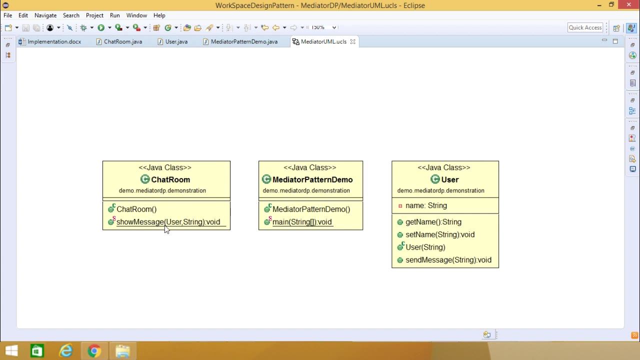 output we are getting. so that is getting printed. and then we are having this name is getting printed and the message is getting printed as it is. so now let us go for the uml diagram. so this is our class diagram here. so here, at first, we are having this chat room. you can find that we are having 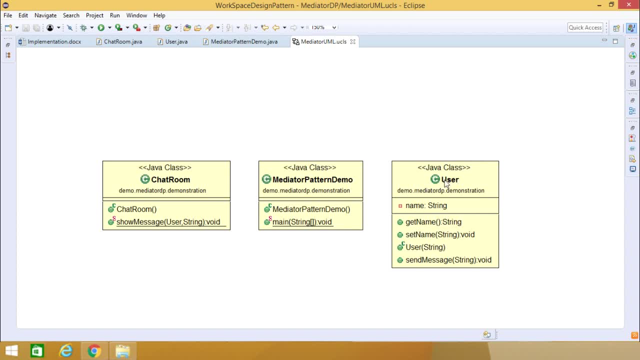 this media, this user class is also there, having the get name, set name constructor and the send message. remember, this show message is of the type static, so static public, public, static, void show message which takes user object and the string as input argument. string object as input argument. 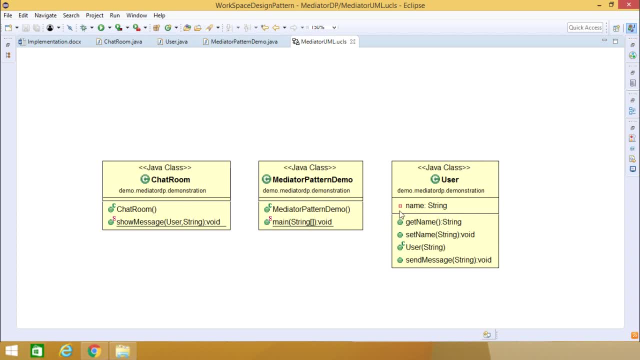 and chat room was there. that is the constructor here. so now here: this name is of the type private, under the scope private and of the type private and of the type private and of the type private of the type our string class. so get name, set name, user constructor and this send message. 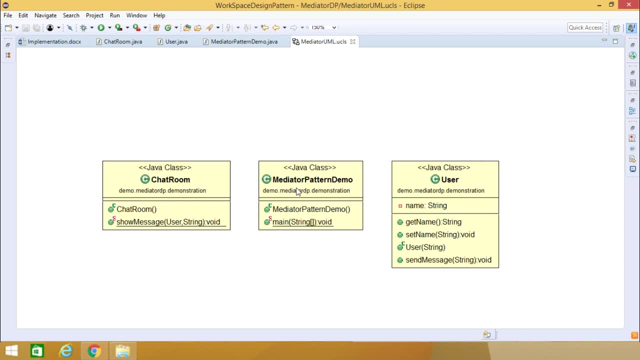 and this is a mediator pattern demo which we executed and we got the required output. so in this demonstration we have shown you that how to implement mediator design pattern using java code. thanks for watching this video.